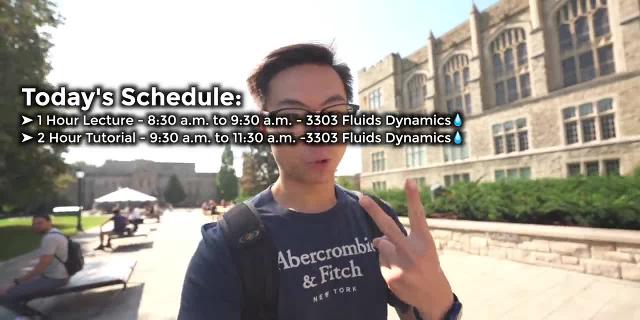 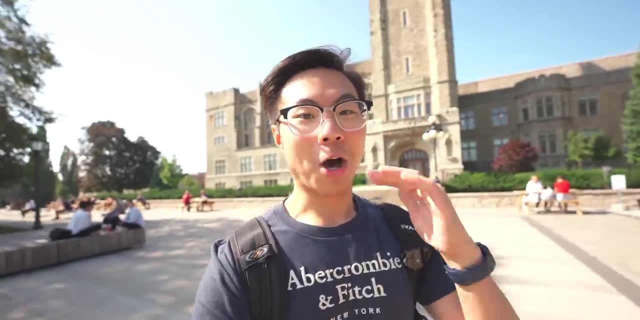 So first I have a one-hour lecture, then a two-hour tutorial and another one-hour lecture, so that's a four-hour block. And then I have a one-hour break, followed by another one-hour lecture, And then, to top it all off, I have a lab. 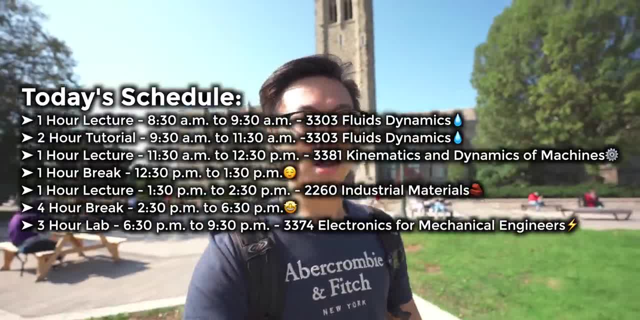 that is from 6.30 to 9.30, so another like hour, Three hours actually. So it's going to be a long day. I really think you're going to like the lab because it's like circuits and stuff. 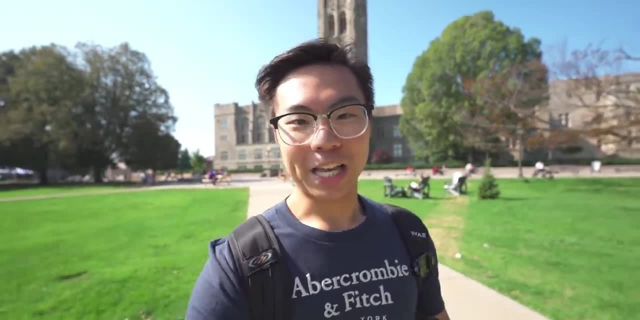 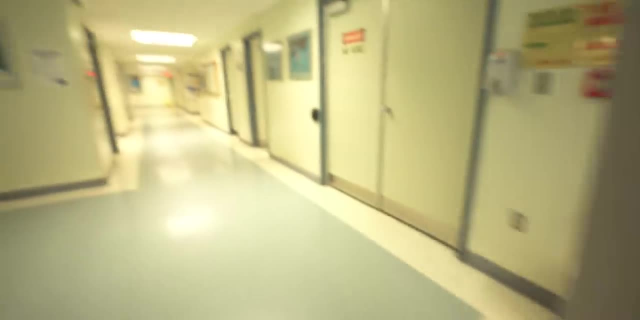 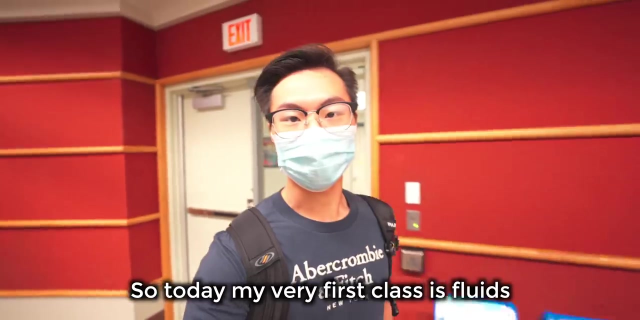 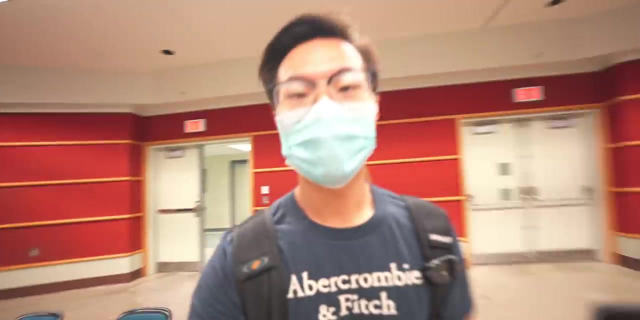 So follow along with me today in this journey. Welcome to a day in the life of an engineering student, And yeah, So today, my very first class is fluids and I'm in this giant lecture hall. Cool, Let's grab a seat. 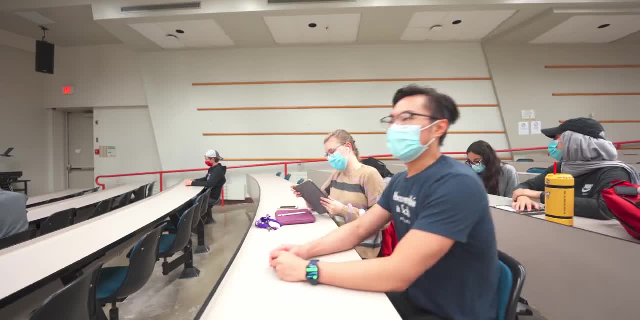 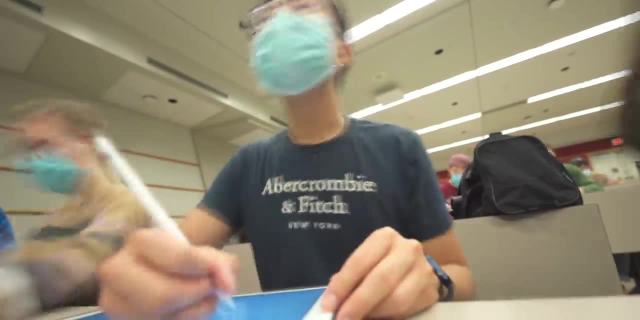 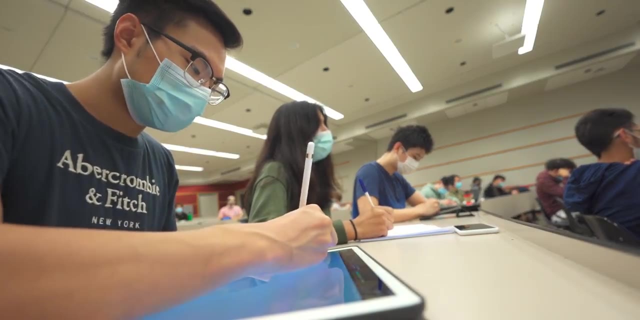 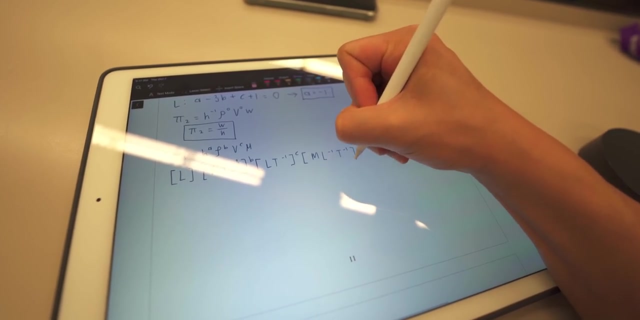 We can make it together. What goes up must come down. There's lots of friendly faces all around And nothing's ever looking behind A little touch of your sweet desire, While we're all looking right. Wait, what's going on? I need a coffee because I'm going to die. 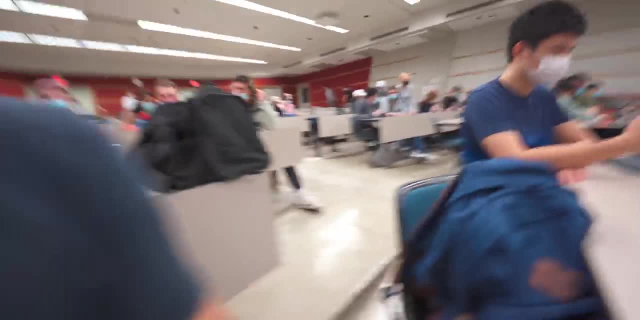 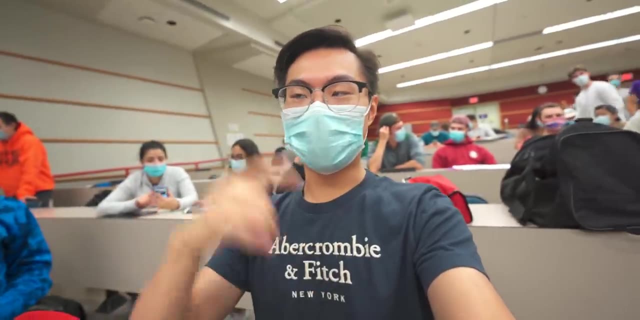 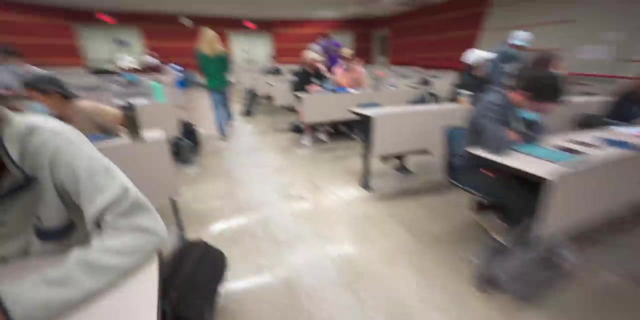 Tim's Alright. so now we are taking like a five-ish minute break in between now and a tutorial and my buddy, Shreya, is going to get some coffee for all of us, because I really need that right now. What's going on, buddy? 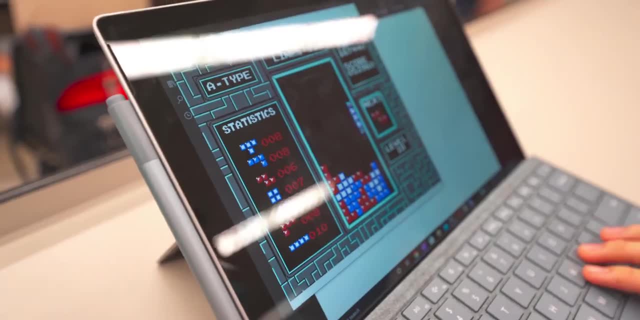 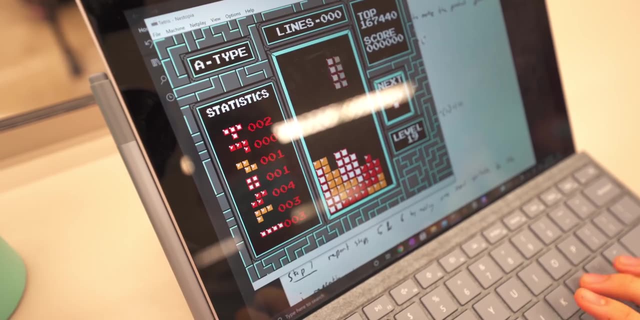 Yo, Yo, Is that Tetris? Yeah, Let me give this a try. Okay, let's see you, and then let's see me. Yo, this guy's actually, This guy's actually like really good, Alright, your turn. 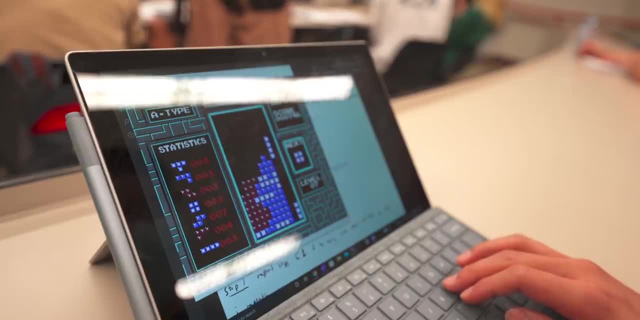 Yo, look at that break, bro. No, you're killing it. Oh, I miscalculated. Oh, no, Okay, no, no, you're ready. you're ready, Wait, wait, wait. No, I messed up. 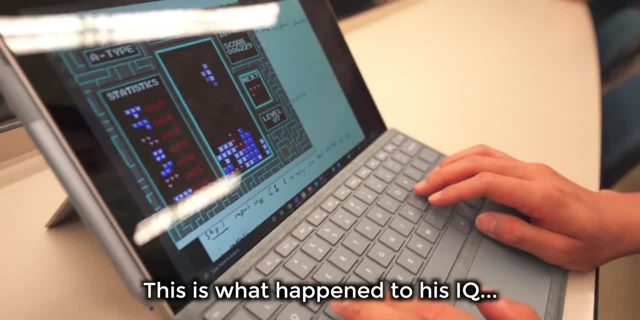 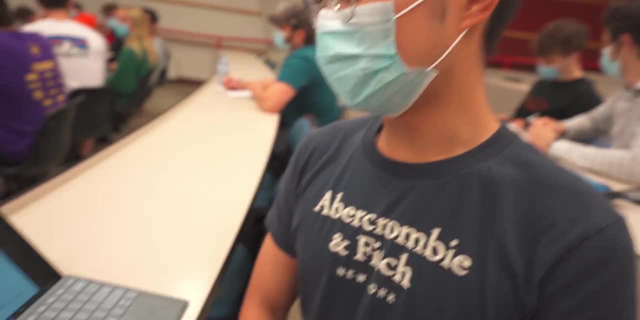 I messed up. A university student played Tetris for a week. This is what happened to his IQ. Bro, where are you going to get that? I don't know. Oh yo, Oh, my god. Yeah, Tetris is uh, more of this guy's thing. 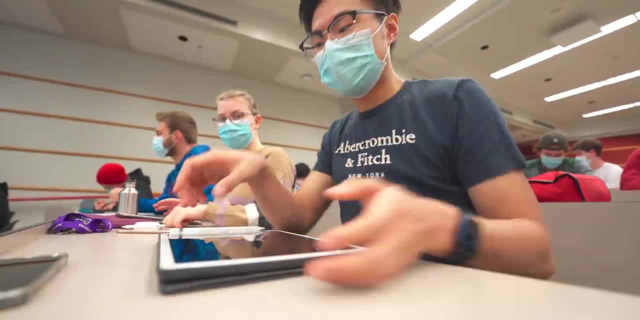 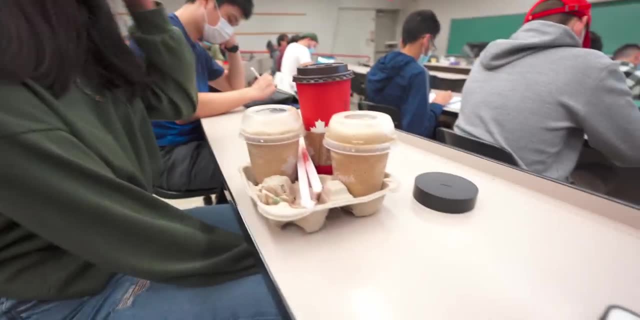 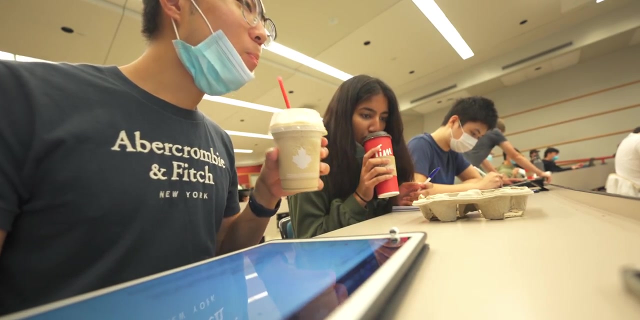 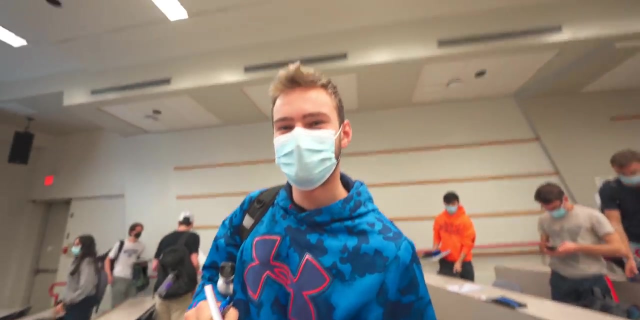 I'll carry you So tenderly. What I wanna say is that Yo actually thank you so much, Father. When the river is calling, I said I love you. I wanna see myself in that vlog. Hell yeah, Yo. let me ask you a quick question. 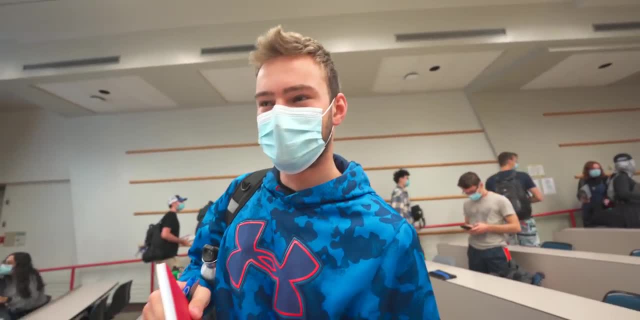 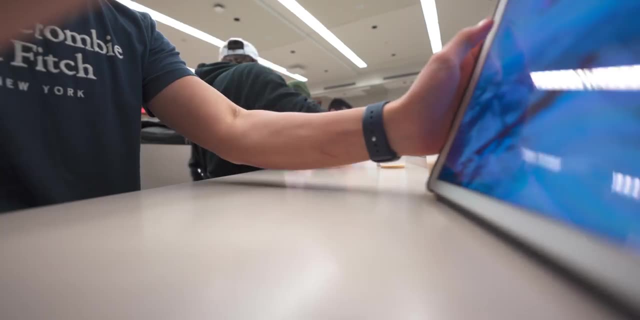 What has four wheels and flies Garbage truck. Yeah Yo, Too many questions. I can never say it. Go on, Okay. so now we're going to get a tour around the stadium. You know we are going to have a good time. 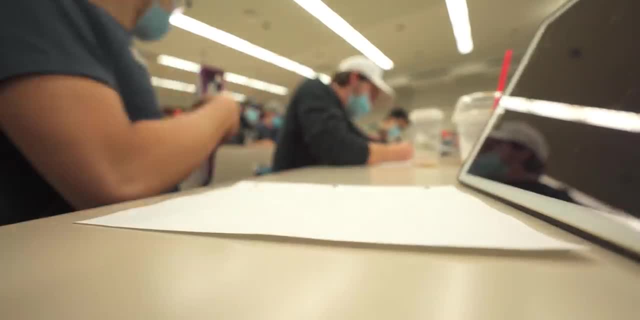 We are having a great time. We're going to have fun. We're going to have a great time. I'm gonna go to the gym, Thank you, And I'm gonna stay here and watch the video. Okay, Oh, no, Okay. 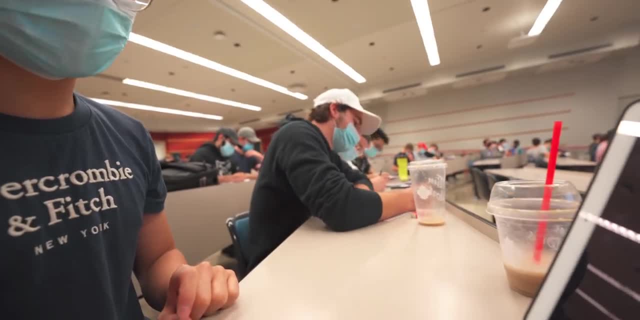 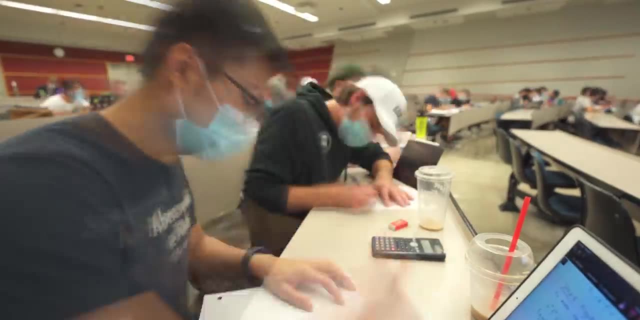 You are going to have fun, All right, We're going to have a nice lunch. I want a drink, Oh right, You guys are working out. Yeah Yeah, I'm gonna have a drink, Oh okay, This one is for you all. 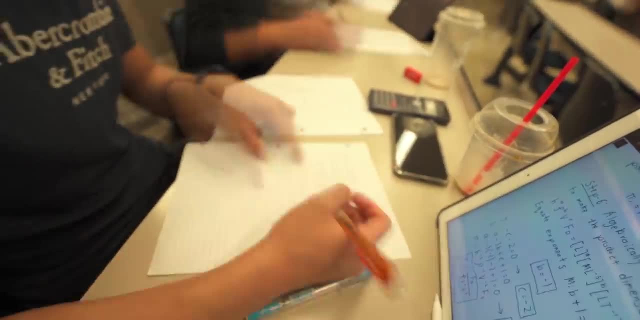 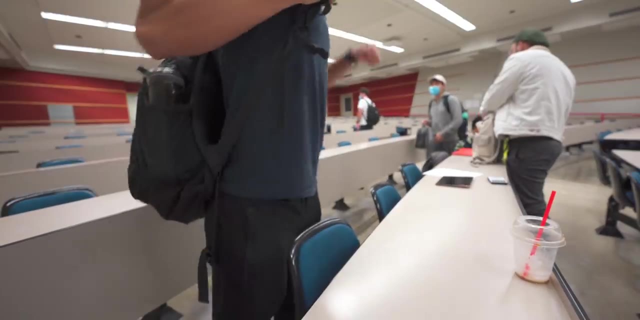 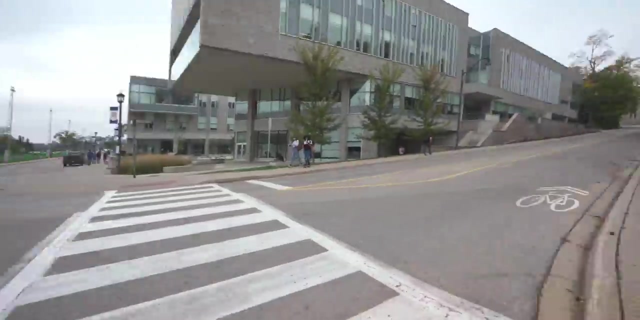 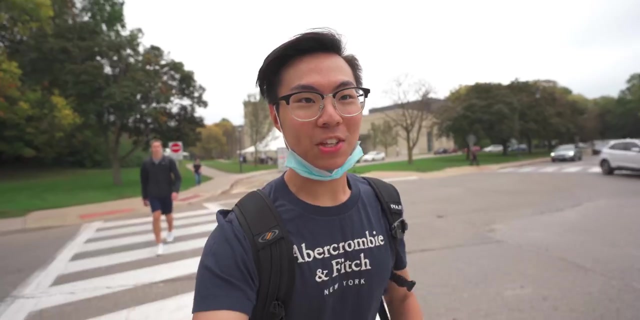 Okay, thanks, This is for you. Okay, now let's go to our next class. Okay, so we finished our one hour lecture and our two hour tutorial, So that's three hours done so far. We still got another hour in our four hour total block. 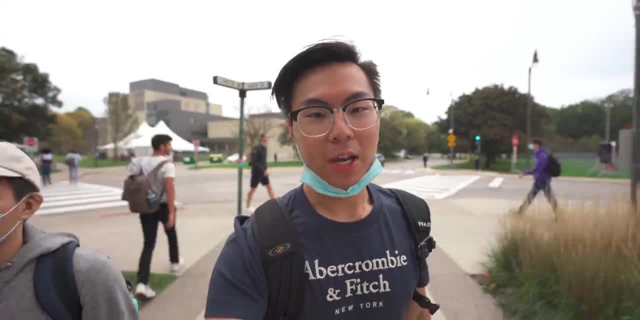 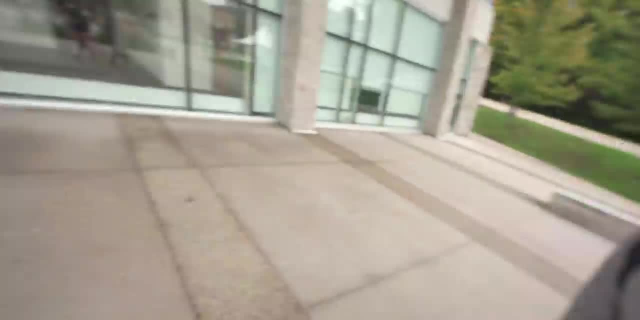 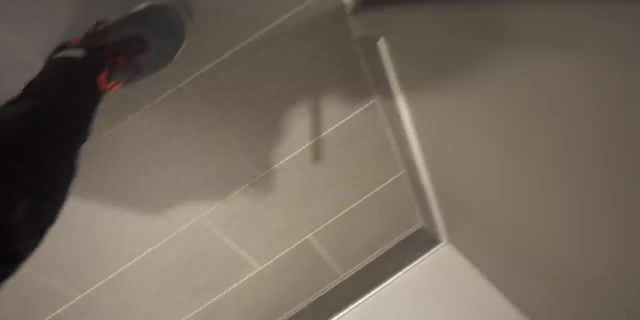 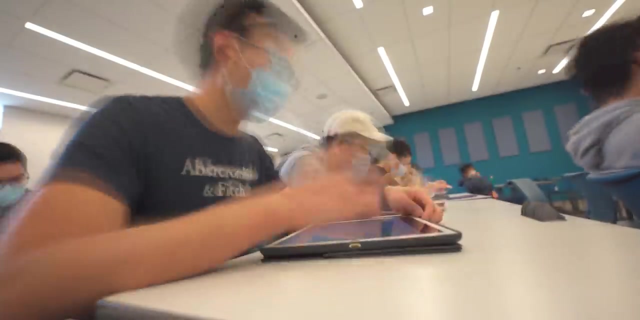 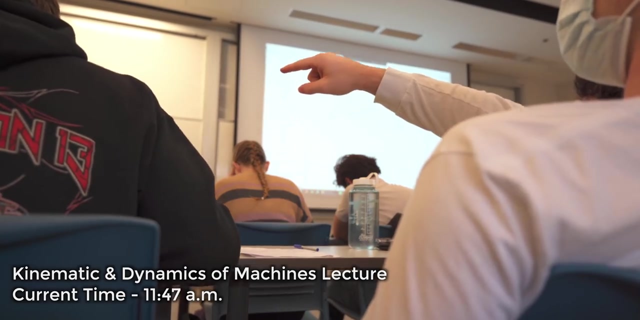 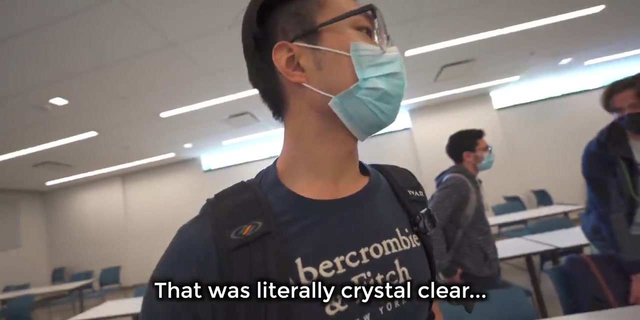 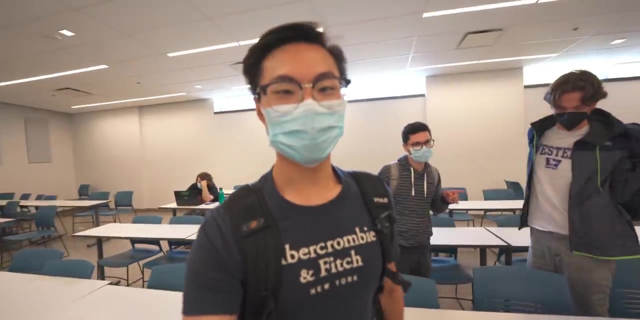 And right now we are going to 3381, Kinematics and Dynamics of Machines, Mechanics, something like that. So, yeah, let's go ahead and do that. We're kind of late, though, Okay, so we just finished technically our second class, So four hours done. 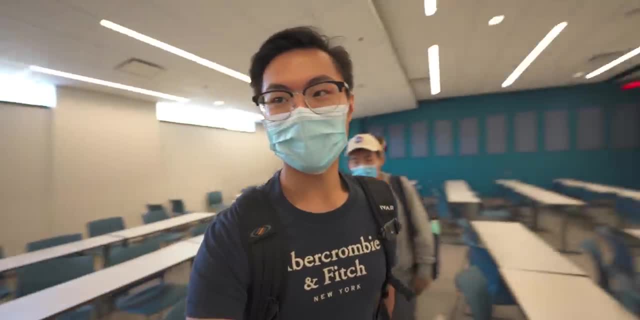 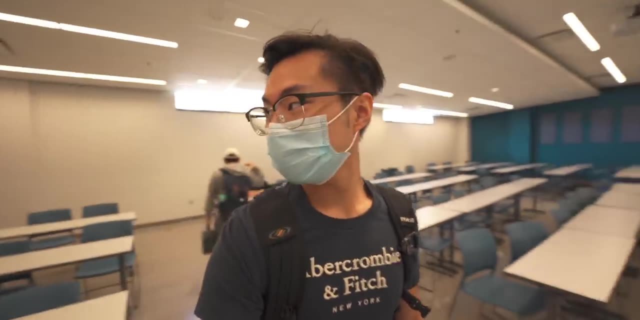 Now I have a one hour break, and then I have one more lecture And then I'm going to have a three hour lab from 6.30 to 9.30. So I am not excited for that. Okay, I think I'll grab lunch right now. 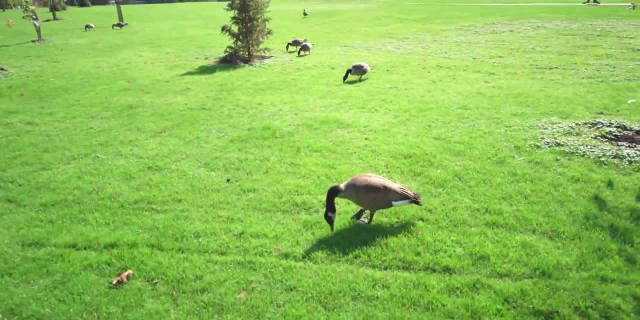 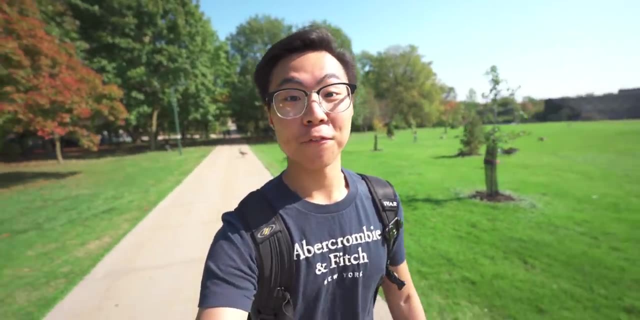 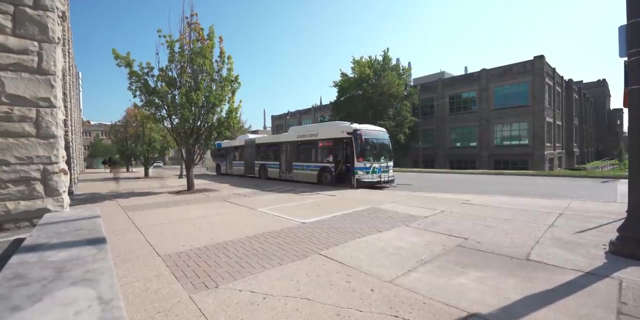 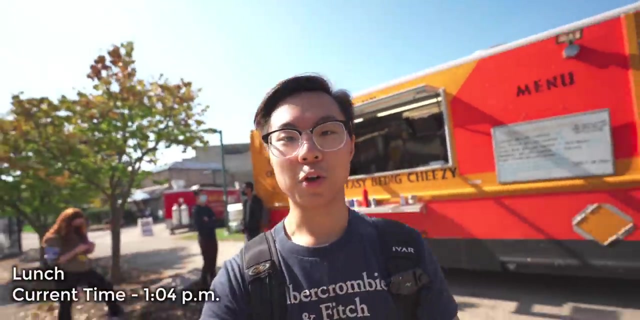 Yo, sometimes I wish I could just be a Canadian goose, So that I don't have to give a single flying Hi. can I get a classic grilled cheese please? No worries, take your time, Okay. so there are a bunch of food trucks over here. 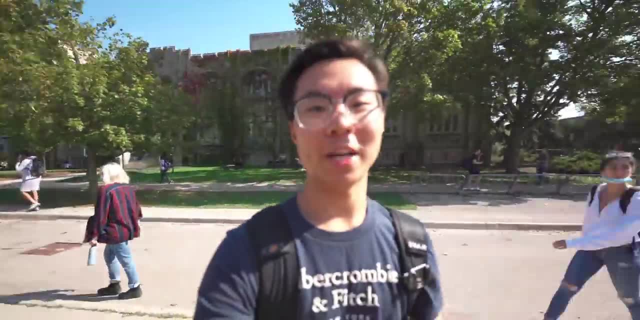 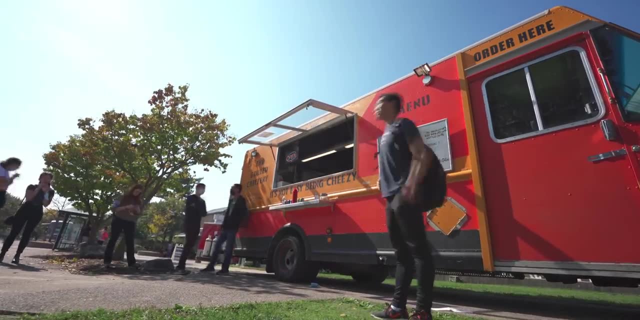 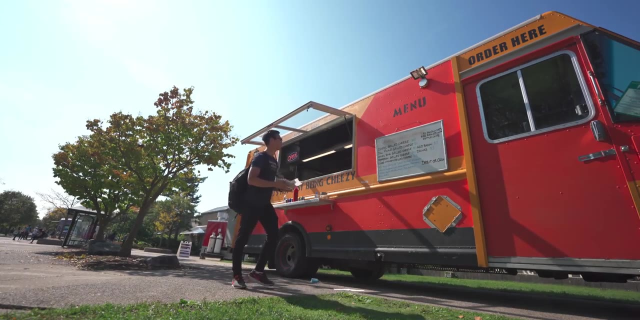 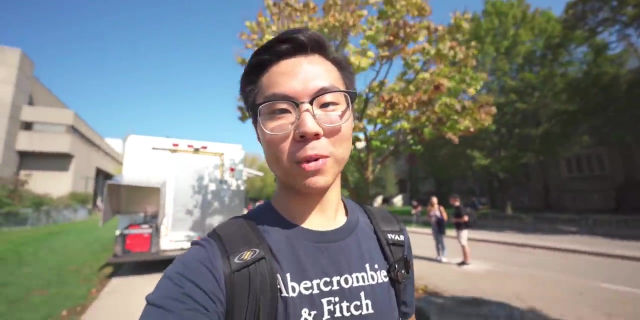 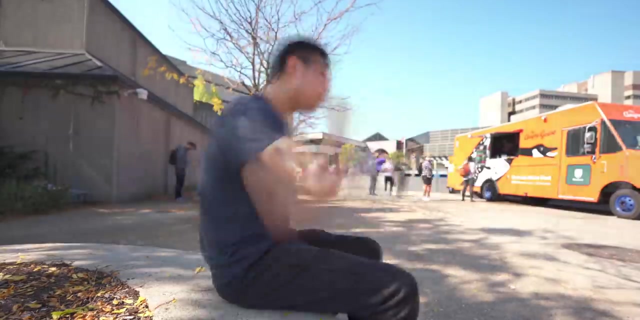 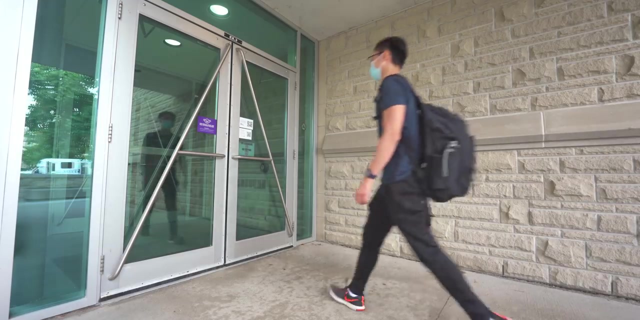 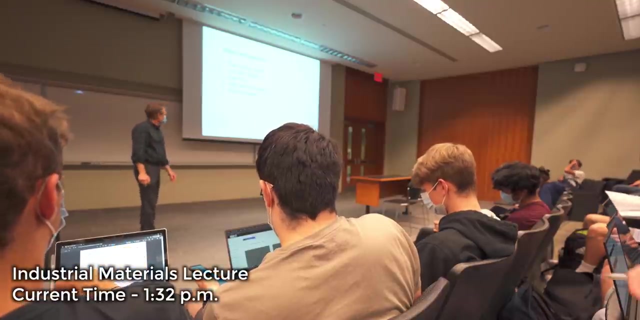 As you can see. Okay, So I decided to get a classic grilled cheese, Because that sounds really tasty right now. Alright, let me just quickly speed around this grilled cheese And then we will head to my next class. All right, let's go. Different types of alloy steel. 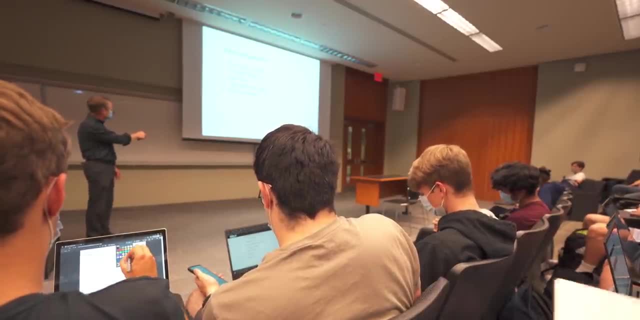 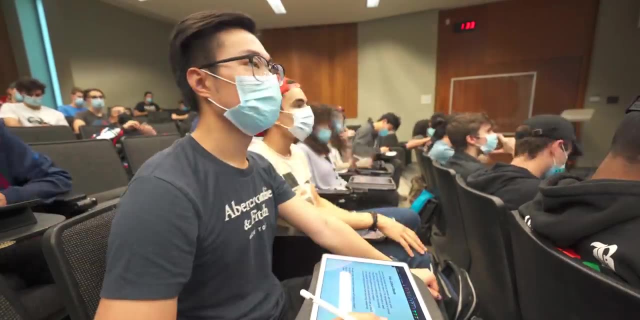 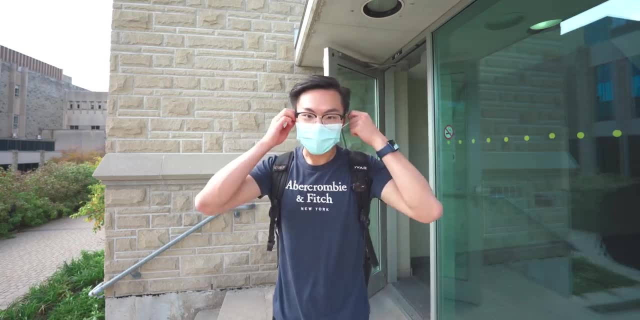 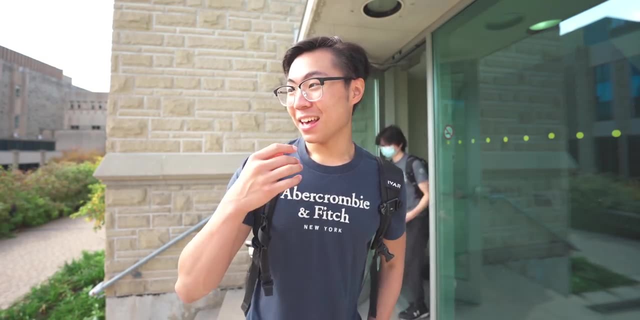 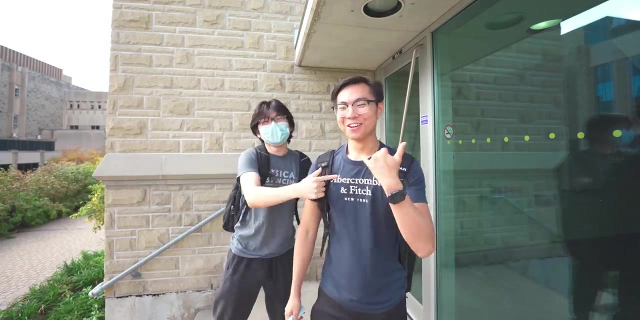 Let's go, Let's go, Let's go. Okay, so I just finished, technically, the third class of today, which is industrial materials. right now I have a four-hour break until I have my. No way, It's J City. It's J City, bro. 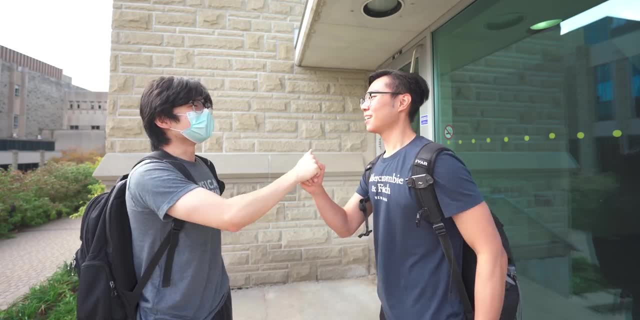 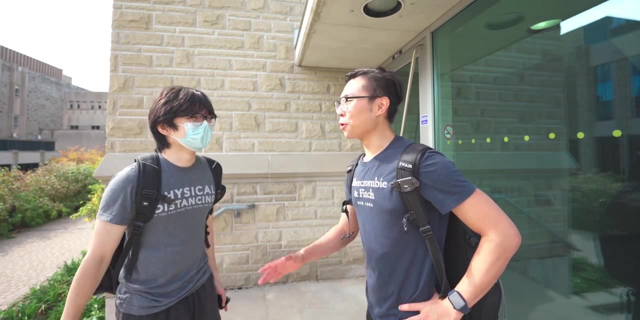 This guy's famous. You're my idol. I met you the other day at Foco. Yeah, yeah, I'm Jeremy. Good to see you, Jeremy. No, no worries, no worries, Jeremy. thank you so much for the support. 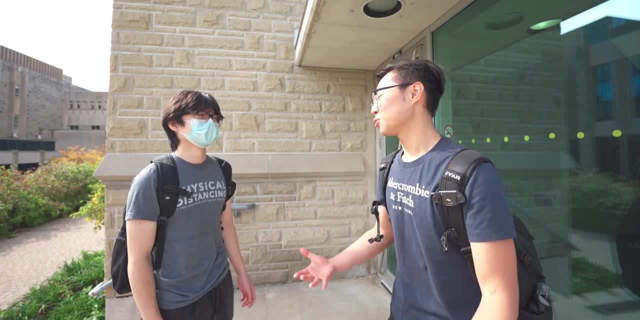 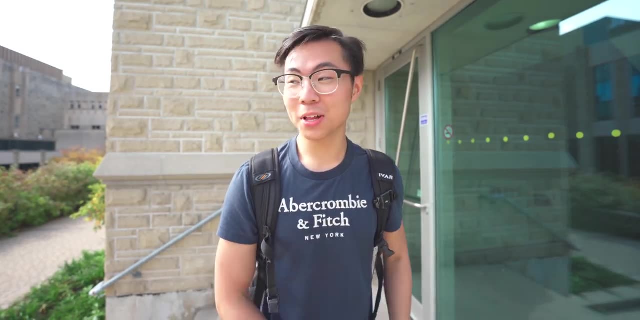 I really appreciate that. Like, you even know how much that means to me. Like, thank you so much. Take care, Jeremy. Okay, so I just finished my last lecture of today. Now I have a four-hour break until I have my three-hour. 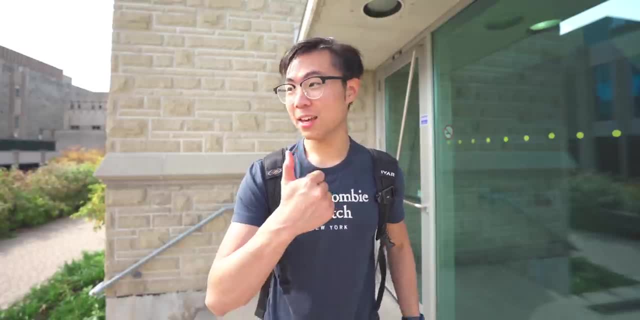 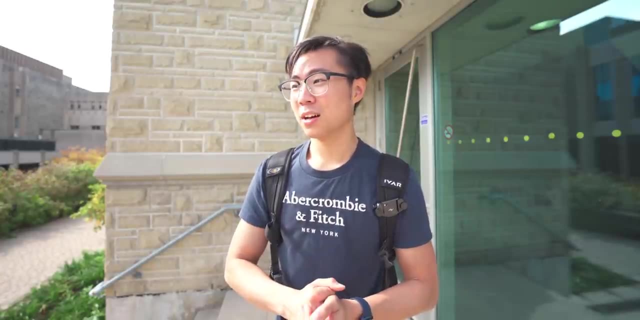 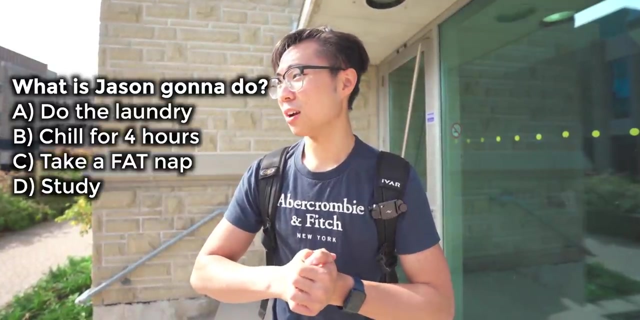 electrical circuits lab. So right now I can either A do the laundry, number two chill for like four hours or three. I can like take a fat nap. so what am I gonna do? I could study too. Option four: 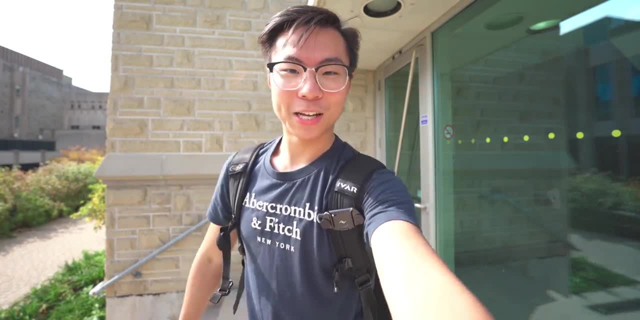 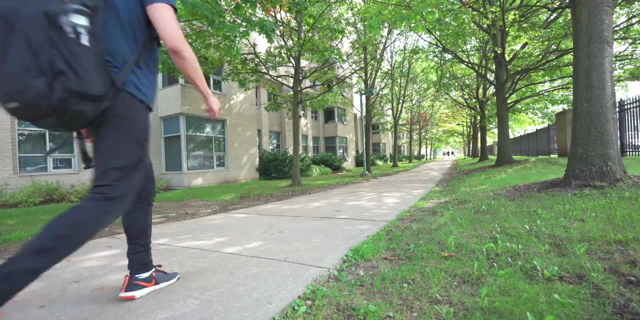 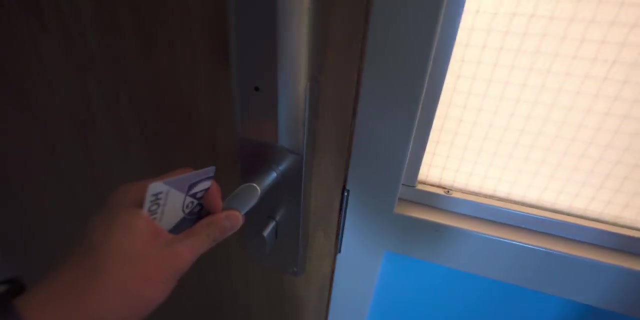 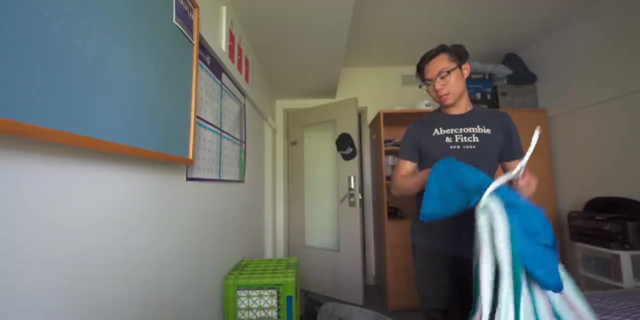 Okay, I think I'm gonna do the laundry and then I'm gonna take a fat nap. That's what I'm gonna do. I actually went swimming for the first time in like years, like two days ago, And I think I will also. 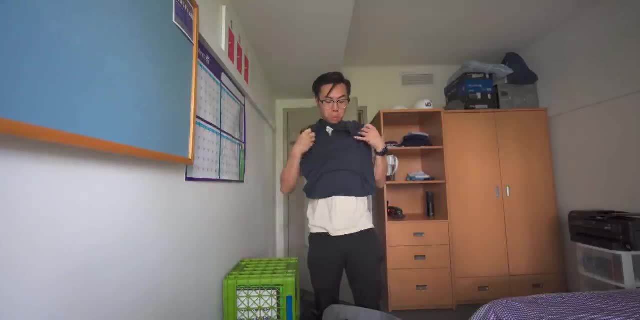 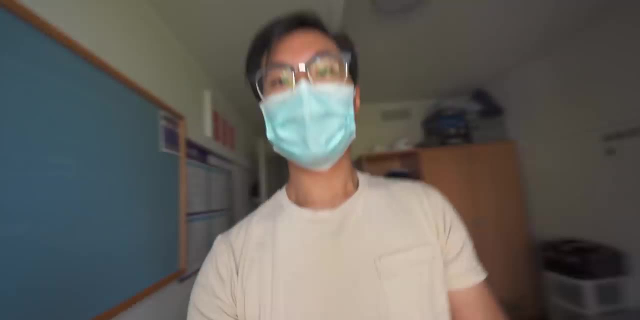 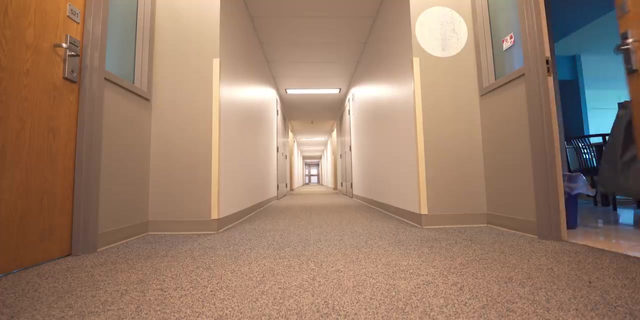 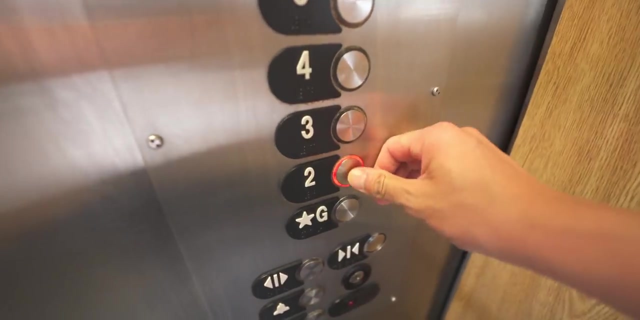 change my shirt, Okay, so laundry is on the second floor of my residence, so I'm going to head to the second floor right now. I wanted to show you guys the laundry process because you know that's also part of the university life. 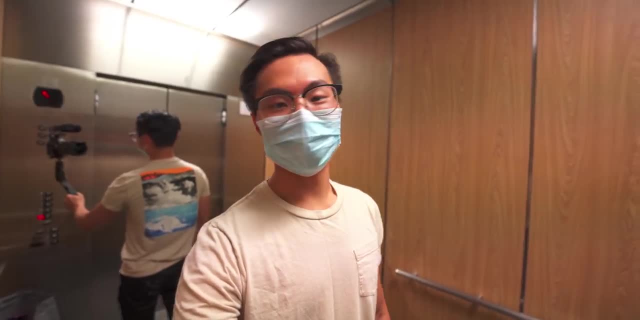 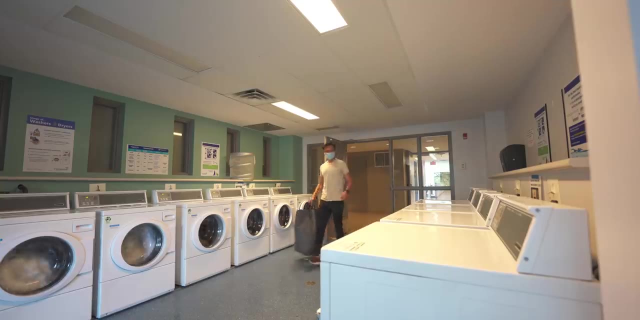 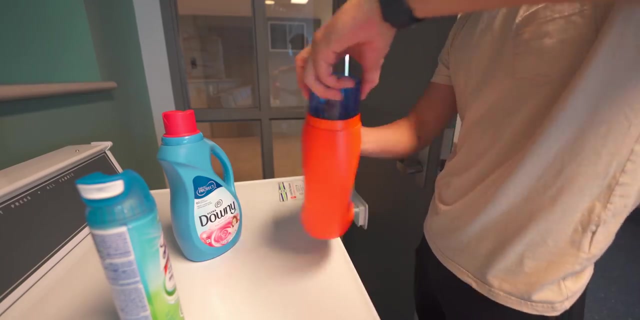 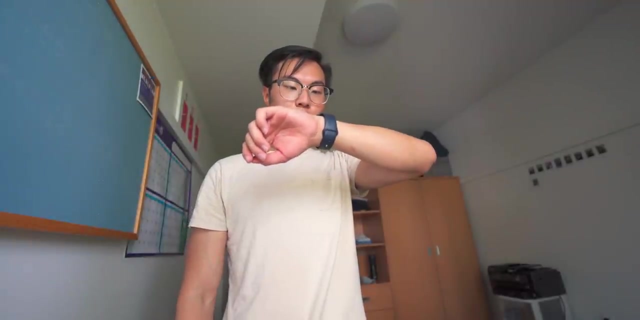 You gotta do like chores. you have to wash the dishes and cook if you have a kitchen. So yeah, chores, real life thing. Hey, Siri set timer for 24 minutes. Okay, so I guess right now I'm going to study. 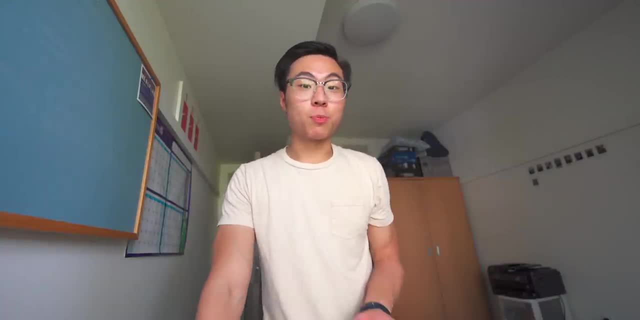 a little bit. Actually, I'm going to work on some kind of like SolidWorks project that I have for design and development, So I can show you a little bit of what that's like. and yeah, here take a look. 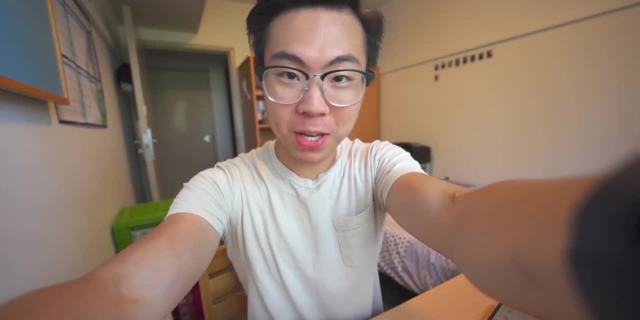 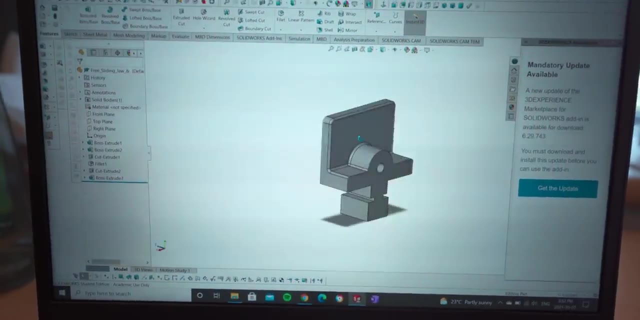 Okay, so this program over here is SolidWorks, and SolidWorks is basically like a CAD software. CAD stands for Computer Aided Design and, as you can see here, this was like a part that was given to us, And I think we have to turn. 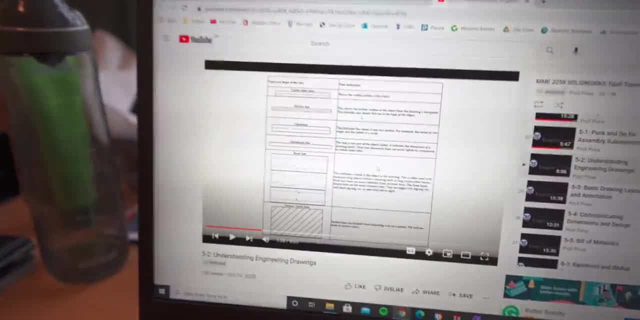 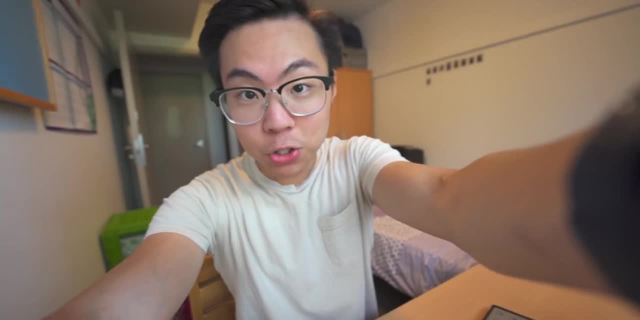 this into some kind of drawing. so right now I am about to watch a bunch of these like tutorials that my professor uploaded and I'm going to watch them. So yeah, if you ever do engineering, then you're going to work with a lot of CAD software. 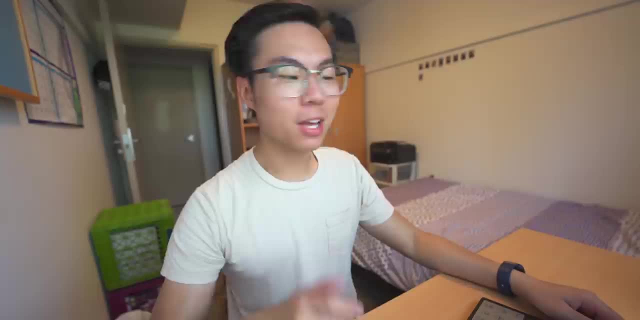 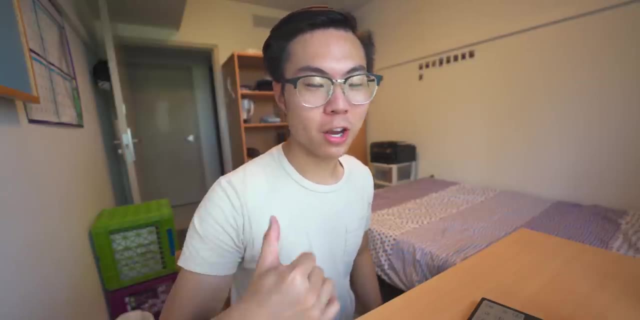 unless you're doing like software or something like that. But if you're in mechanical or Tron, then definitely you're going to have to work with SolidWorks. So yeah, apparently my laundry is done, so I'm going to go put it in the dryer. I'm not going to show you. 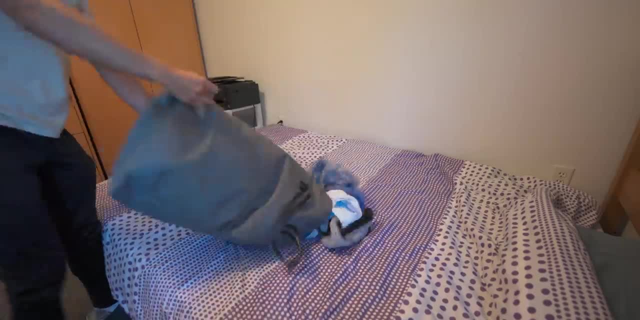 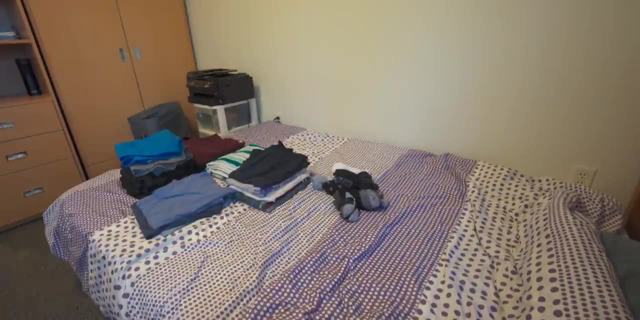 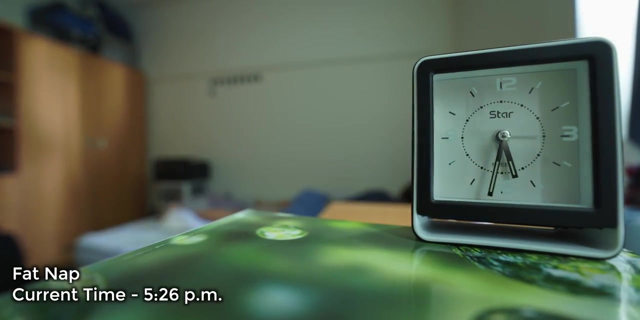 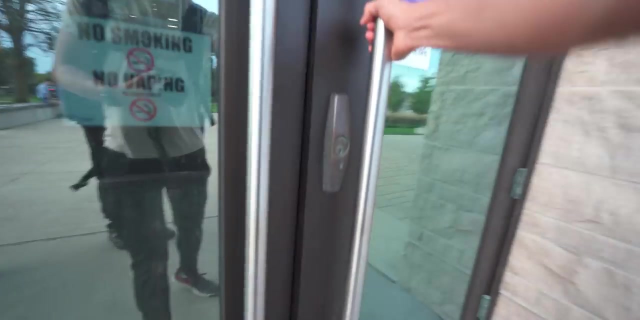 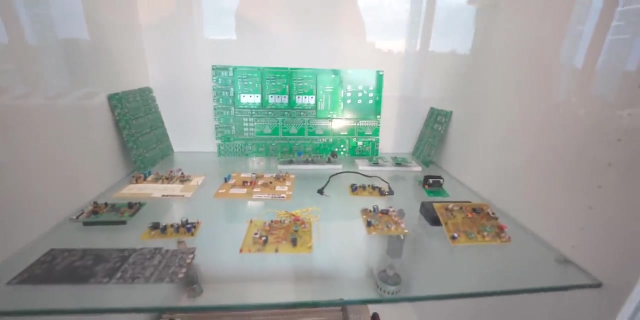 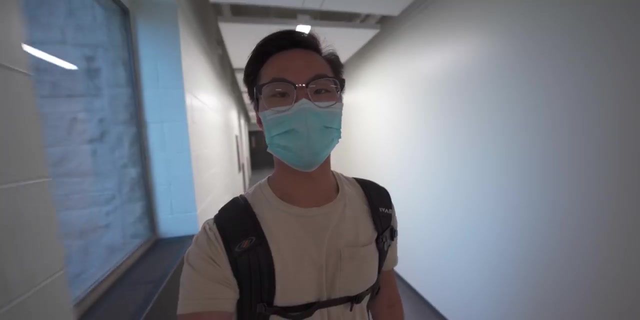 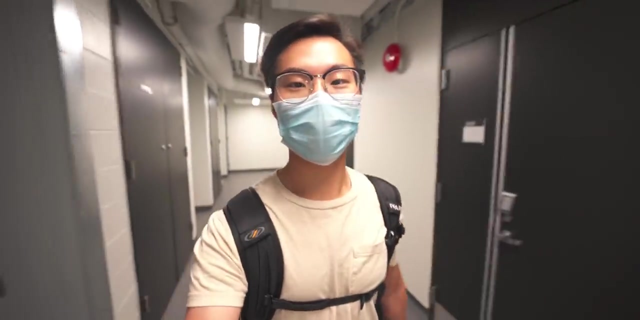 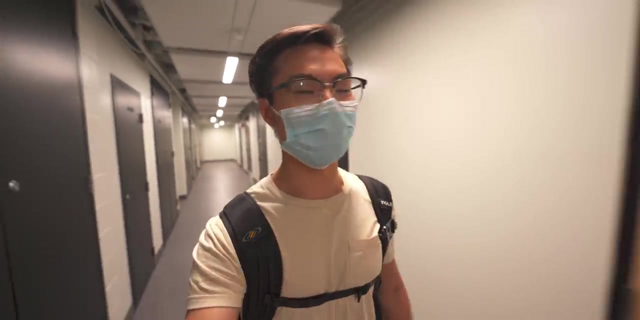 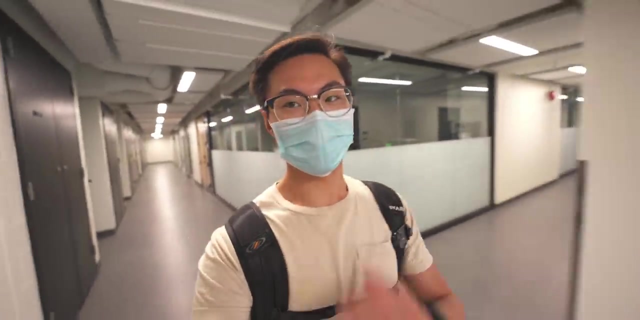 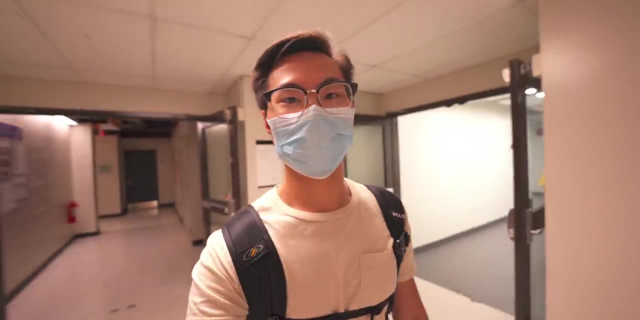 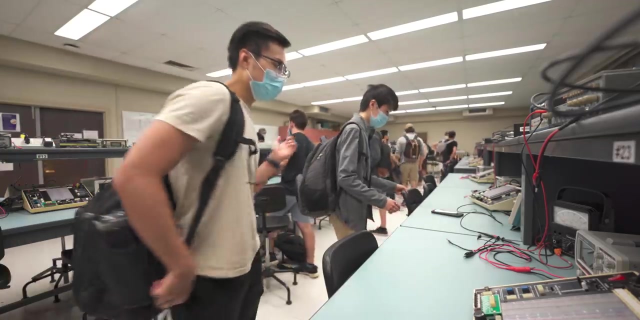 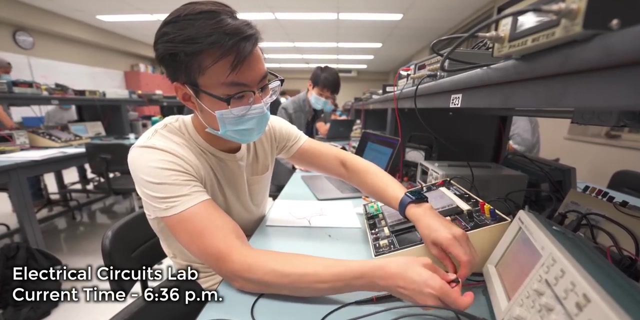 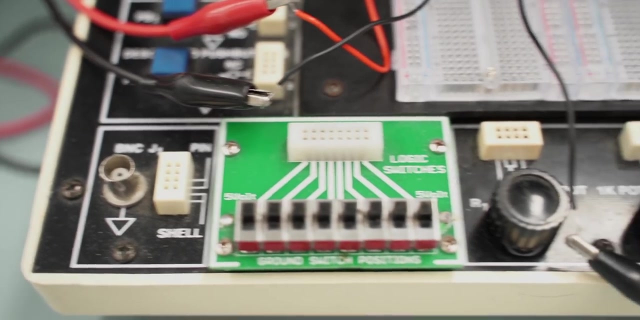 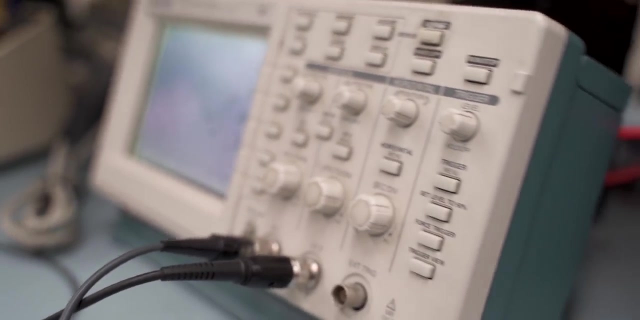 because it's just like kind of boring. but I'll be right back. 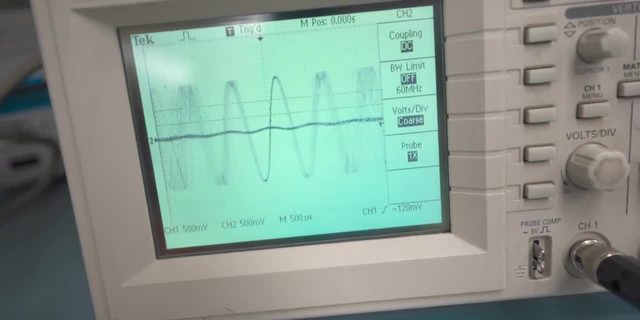 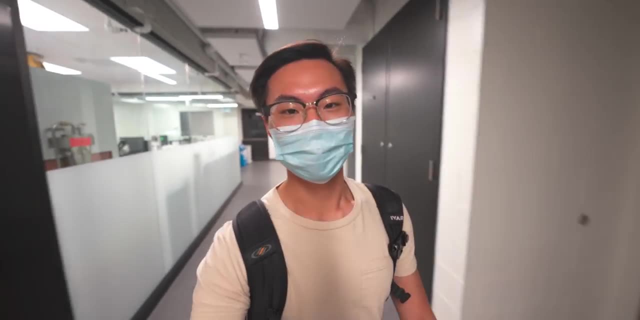 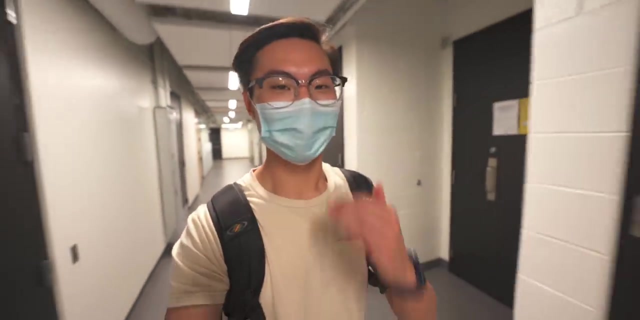 Okay, so I finally completed my electrical circuits lab. I'm really glad that the TA allowed me to film in the lab so that I can show you guys what it's like in an engineering lab. I'm going to. 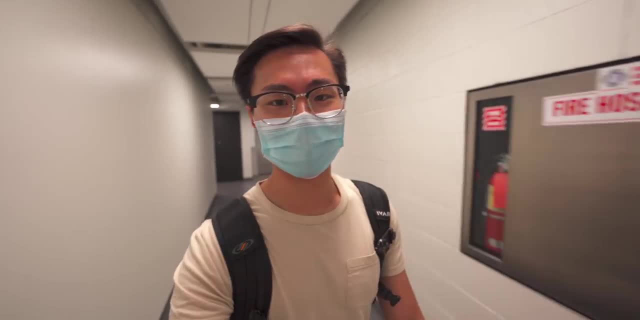 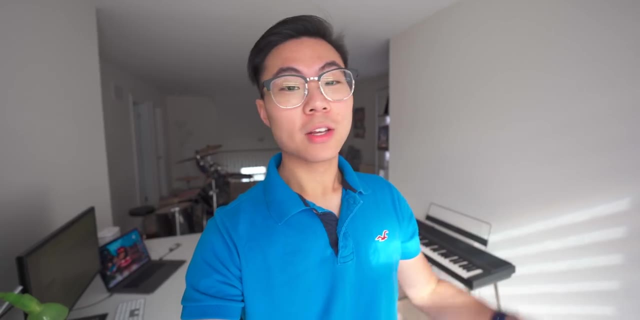 study. I might go to Subway and grab some dinner, because I have not eaten dinner yet, so I don't know. we'll see Whatever I decide next is going to happen in 3,, 2,, 1.. So I decided to go home. 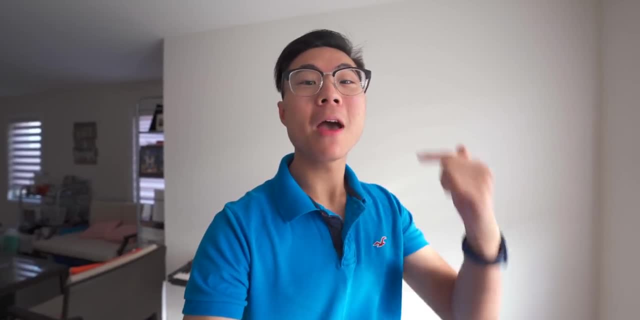 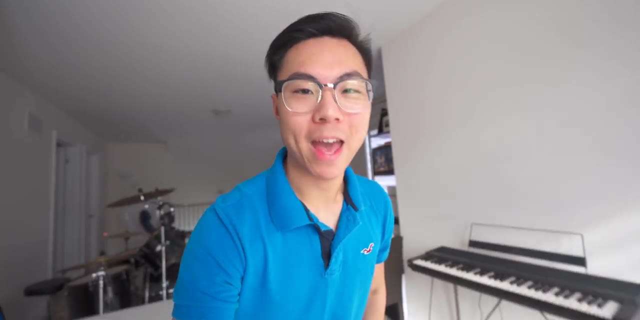 and just sleep, because I was way too tired to do anything productive. but that was actually a couple of weeks ago and I am actually back home for reading week, so hopefully I'll have time to edit and upload this video. Anyways, guys, that has been. 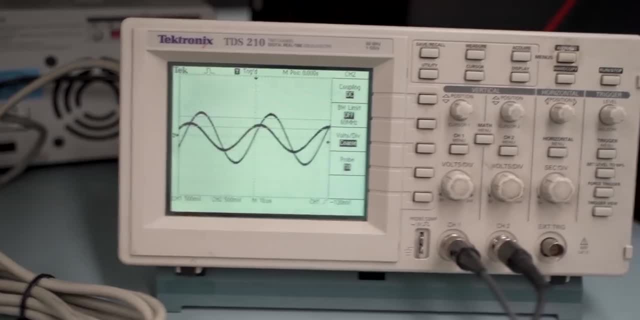 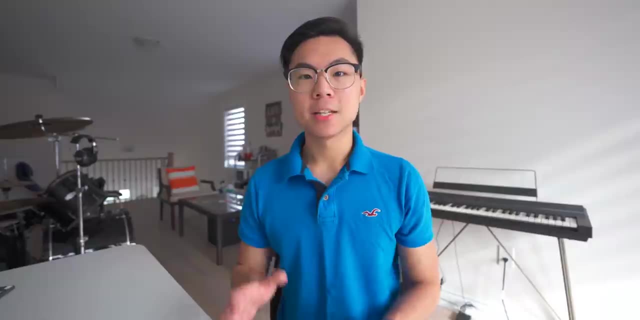 the day in the life of a third year mechanical engineering student. I hope you enjoyed it. As you can see, engineering is an absolute grind, so if you're trying to be an engineer too, prepare yourself. Speaking of, I planned so many videos over the summer that I was. 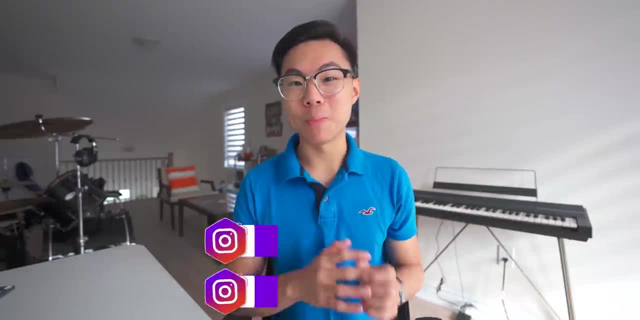 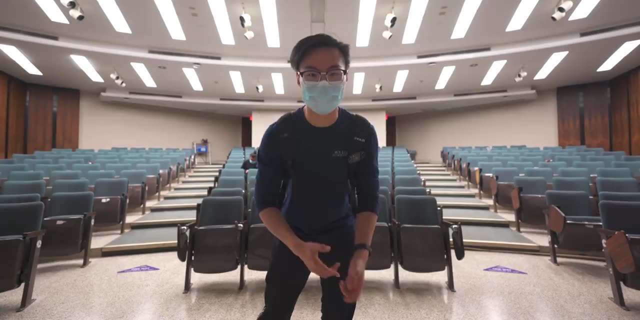 going to make in university. However, I completely forgot how busy engineering is. I have like 6 videos in the bank that I haven't like edited yet, so hopefully I'll have time to edit them during this reading week. If you're new to Jcity, what's popping? My name is. 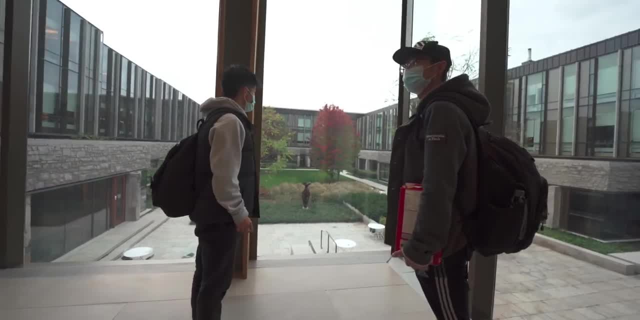 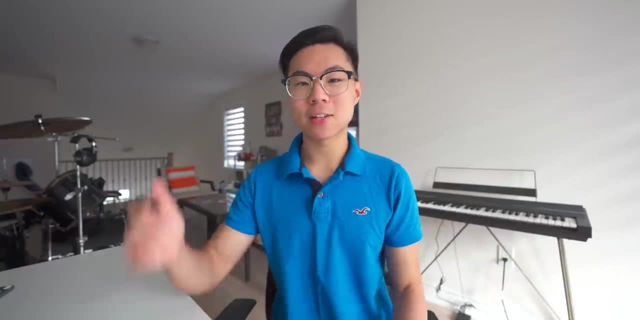 Jason and I'm trying to make more videos showing you my university life while also giving you helpful tips and tricks so that you can survive in university. And if that's your thing, then definitely click that subscribe button and enable those bell notifications, because that will. 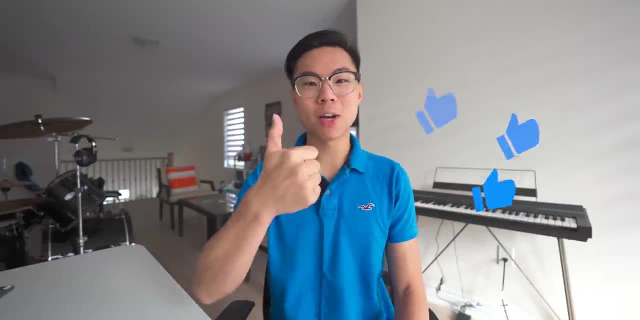 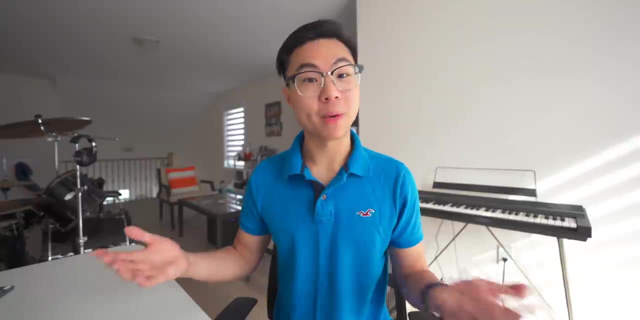 really help me out a lot. And while you're at it, why not give this video a big thumbs up and share your thoughts about this video in the comments below and also let me know what other university type videos I should make next? Oh yeah, if you go to. 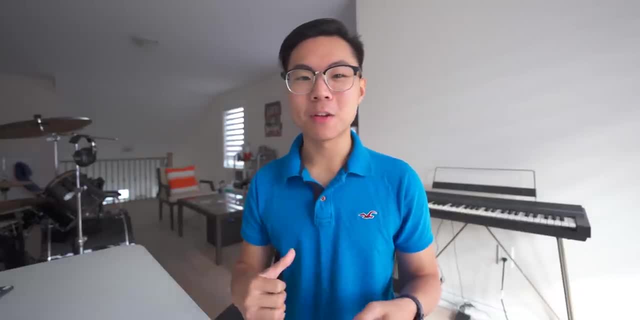 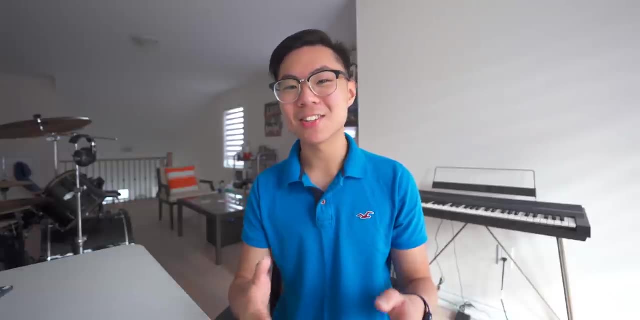 Western and you happen to see me on campus, feel free to come say hi to me, because I am a really chill person in real life and over the past couple of weeks a number of you guys, the Jcitizens, have approached me. 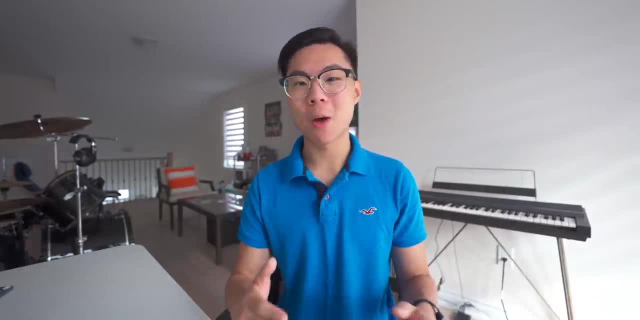 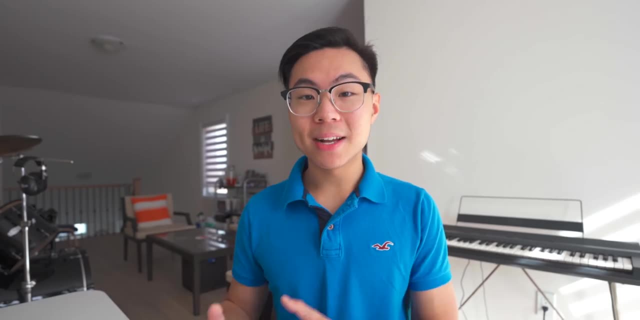 and have said some really nice things to me, and you guys don't even understand how much that means to me. I love meeting you guys in person and your support just means everything, so thank you so much for that. And now that you've made it all the way until: 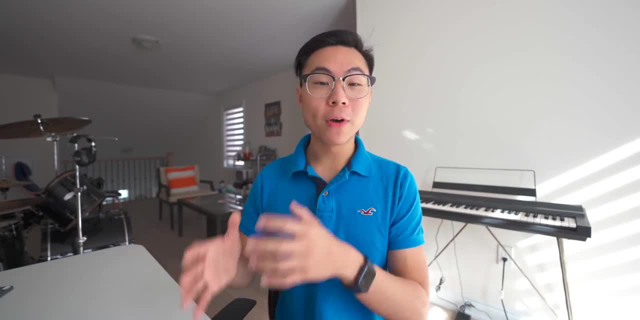 the end of this video. here's a little Easter egg. There's something I've always wanted to try in a YouTube video, but I'm gonna need your help for this one. If you're on a cell phone, this will technically work, but 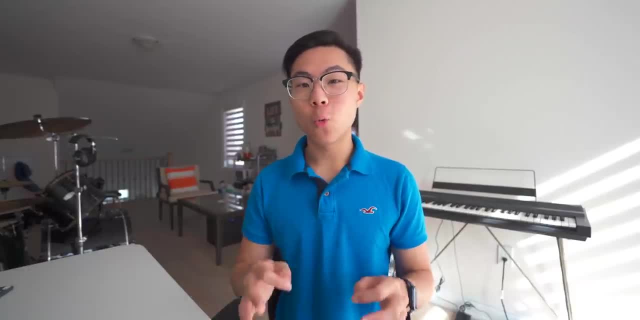 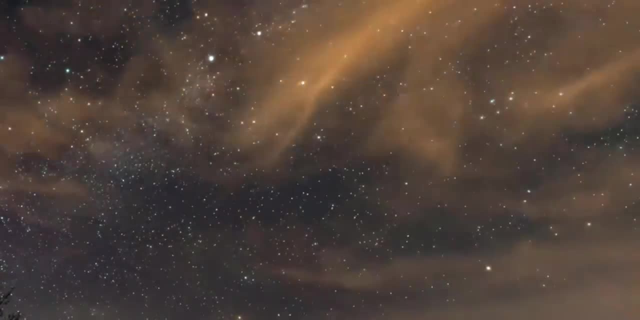 it will work a lot better on an actual computer. So what I want you to do is I want you to loop this video. To do that, you have to right click your YouTube video player and select loop. If you're on a cell phone, you can click the three dots on the top. 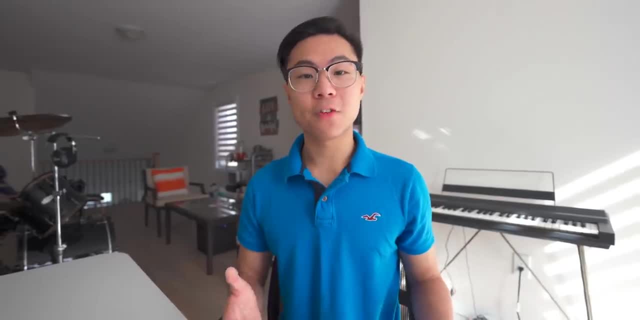 right corner and also select loop. Now that you've done that, let's see if it works Okay.